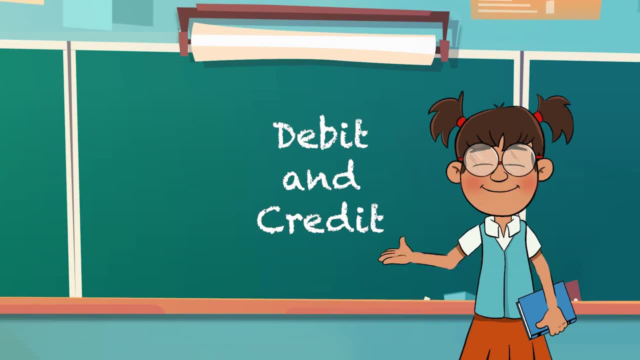 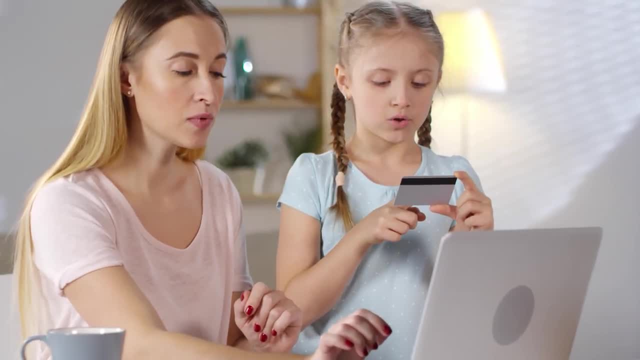 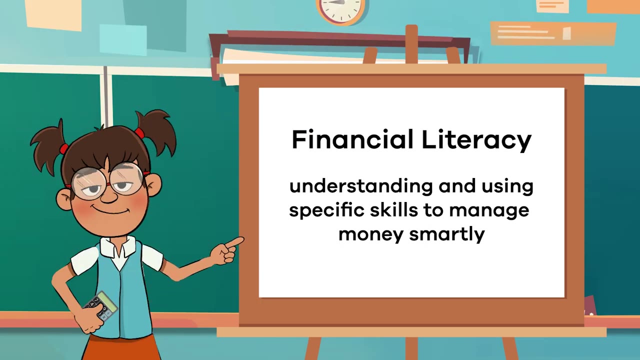 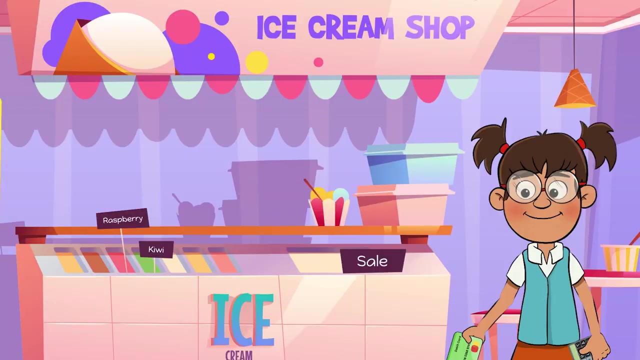 Today we are going to talk about debit and credit and the differences between the two. That way, when you pay for things yourself, you can do so using financial literacy. Remember, financial literacy is understanding and using specific skills to manage money smartly, And understanding how debit cards and credit cards work. 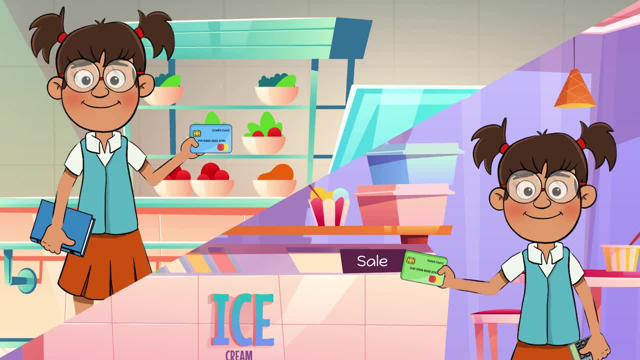 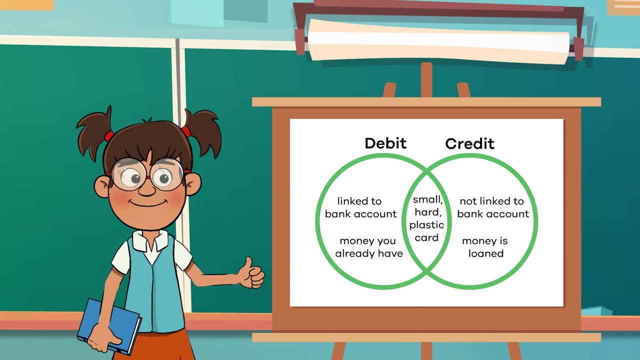 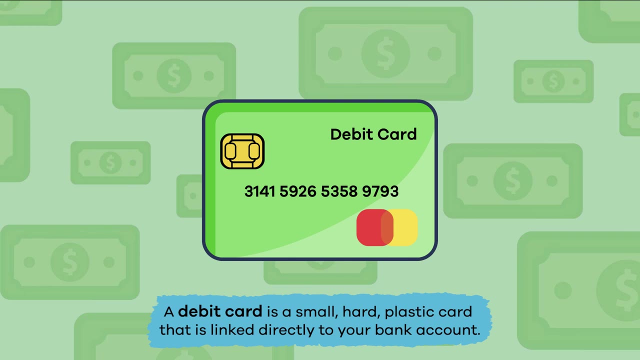 will definitely help your financial literacy skills. So let's get into it, shall we? First, let's talk about the difference between a debit card and a credit card. A debit card is a small hard plastic card that is directly linked to your bank account. 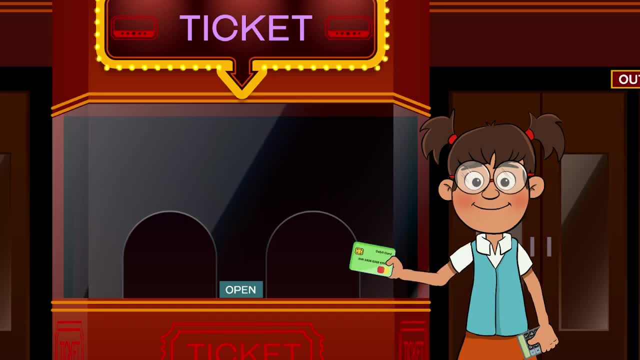 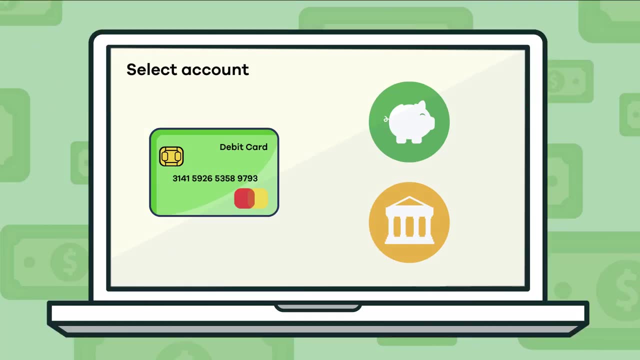 which means you can pay for things using small plastic cards. Second, you use your debit card to pay for things with the money you already have. Most often, a debit card is linked to what is called a checking account. If you do not have, 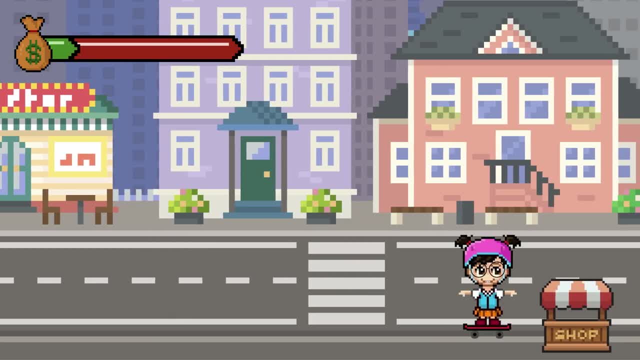 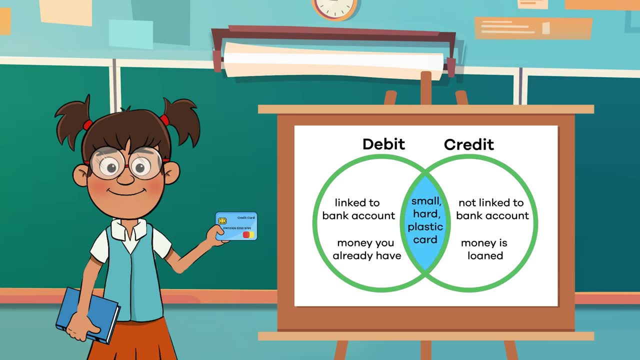 money in your checking account. you cannot use your debit card to pay for things. Even though a credit card is also a small, hard plastic card, it is not linked to a bank account. Instead, a credit card is linked to a small, hard plastic card. Instead, a credit card is linked to a bank account. 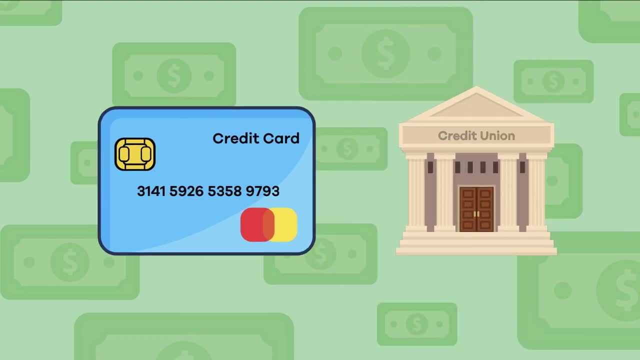 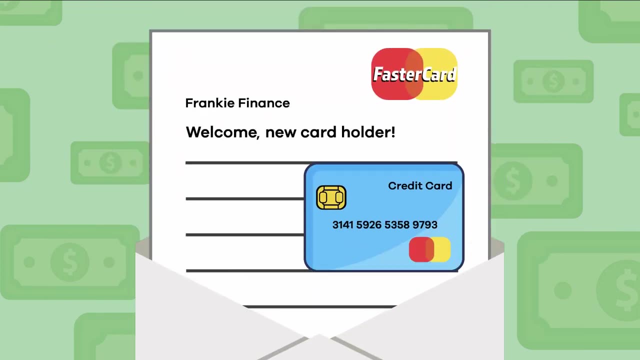 It is done to see what is called a credit card, because one type of雪 is linked to other corresponding kinds of card, or money On the baby of a dollar is dealable currency. In the case where you purchase a card, you are given two different allowed amounts. 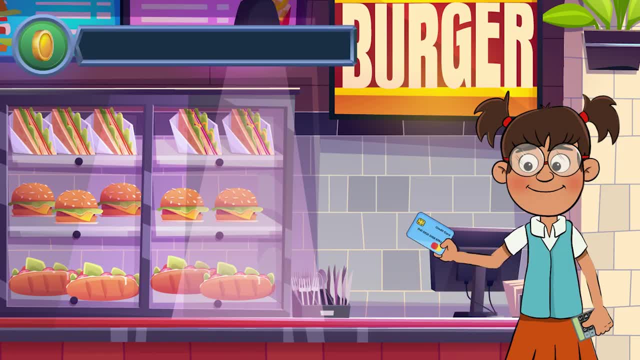 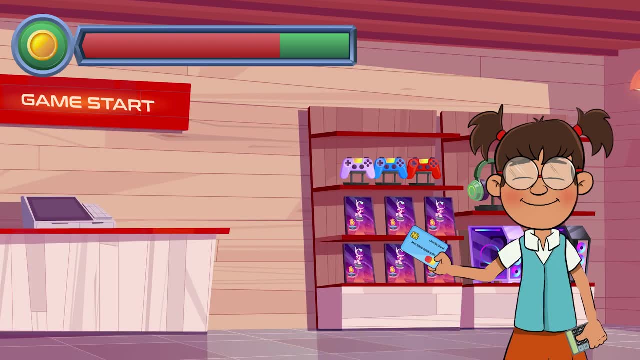 when sending for the card. If you ketchup paper at your phone, you also have to give credit card. customers who install credit card should send a damage to your credit card when sending for their credit card until the payment is given for the card in real time. 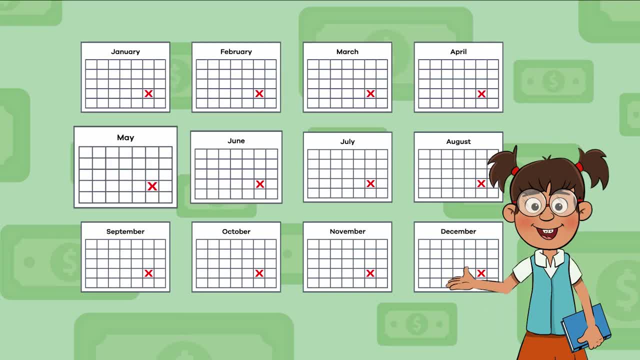 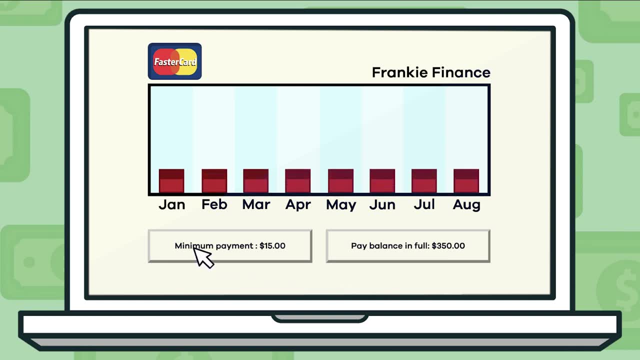 thus giving your credit card to another party again, suff corners and so on. usually one payment per month. Typically, you have to make a minimum monthly payment on the amount you spend, which is the least amount you can pay the lender back each month to reduce your debt. 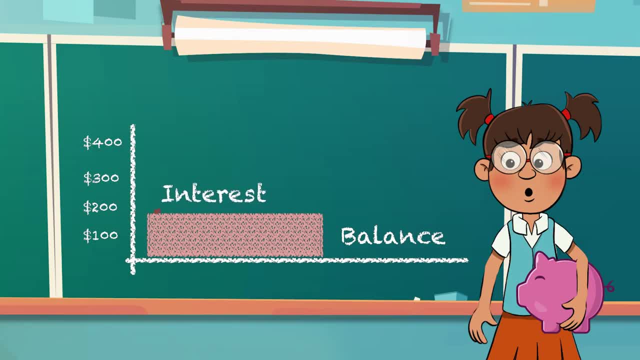 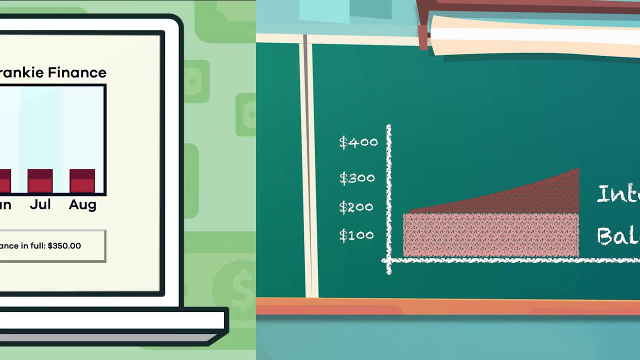 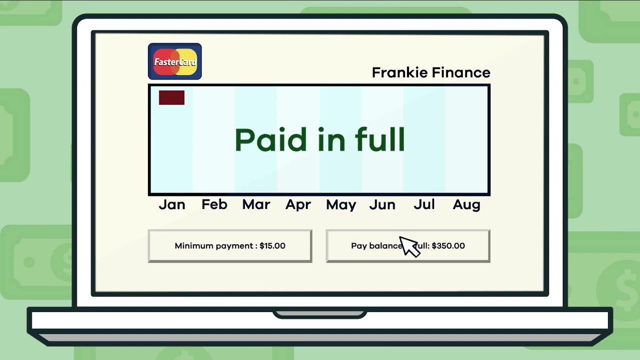 Credit card companies also charge you interest if it takes you longer to pay the money back or if you do not pay the full amount back every month. However, if you pay off all of your credit card balance every month, which is also called paying in full, you will not be charged interest on your purchases. 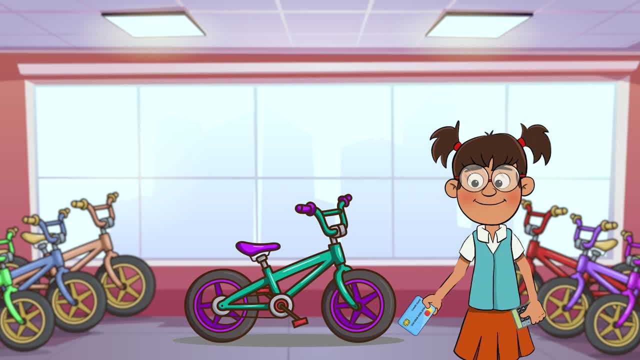 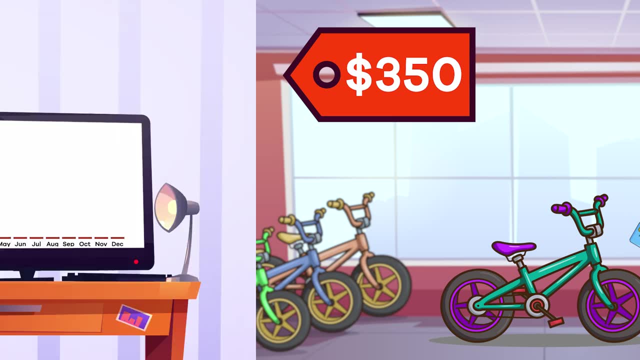 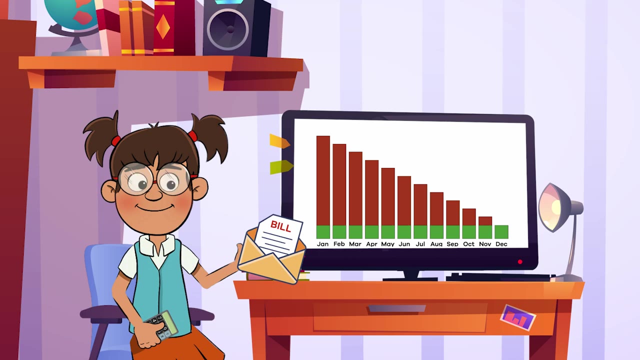 For example, Frankie Finance is thinking about charging a new bike on her credit card that costs $350.. The minimum payment she would have to make each month is $15 until the balance is paid. Paid down to zero. Sounds pretty reasonable, right. 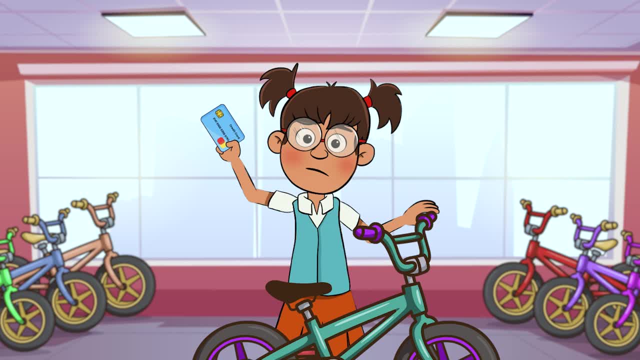 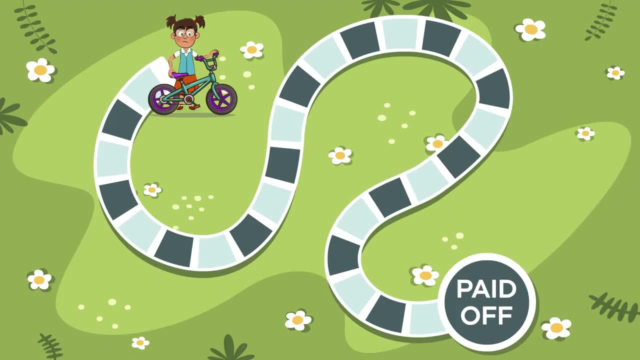 But wait, we don't have all the facts. The credit card company wants to charge her 16% interest on her purchase. At 16%, if Frankie pays only the minimum payment of $15,, it will take her 27 months to pay off the bike. 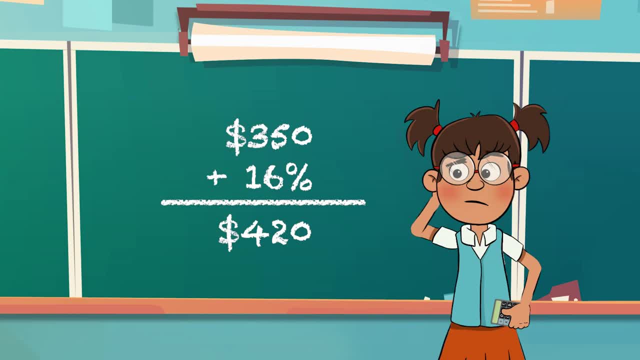 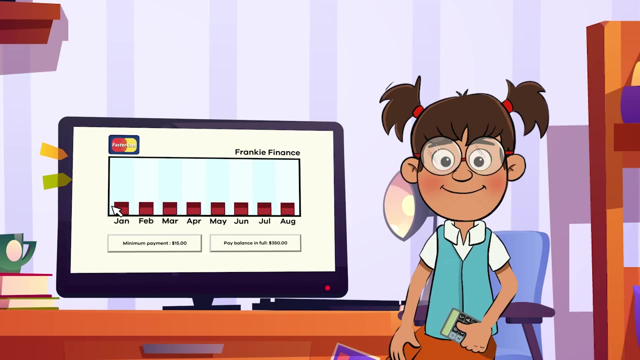 That is, over two years. Not only that, but also if Frankie pays only the minimum payment of $15,. that is a long time, but Frankie would actually end up paying about $70 more for the bike because of interest charges. However, if Frankie is able to pay off the whole amount of $350. 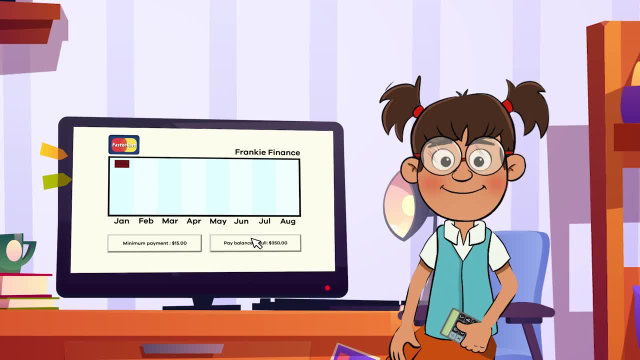 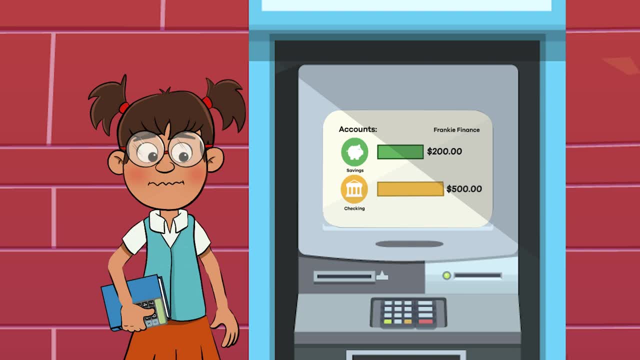 in full that month, she will not have to pay any interest. Frankie also looks at her checking account and realizes that she has $500. She could pay for her new bike in just a few days. But if Frankie pays only the minimum payment of $15,, 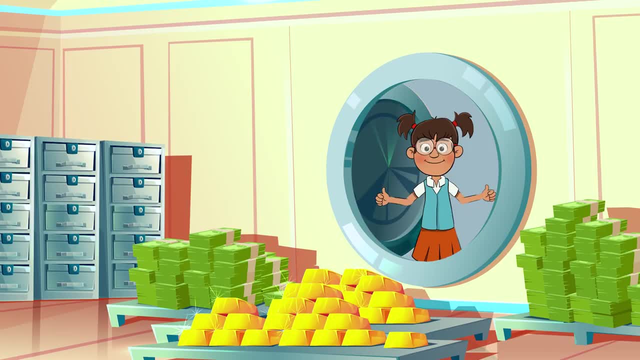 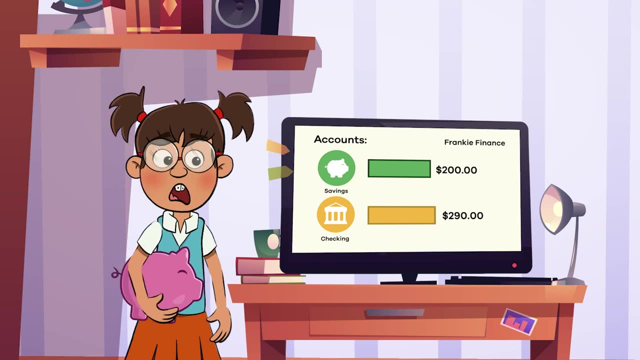 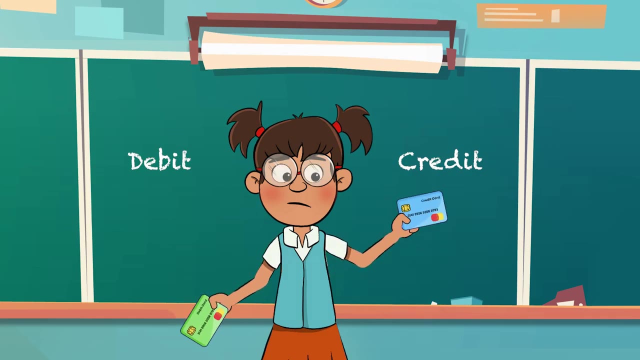 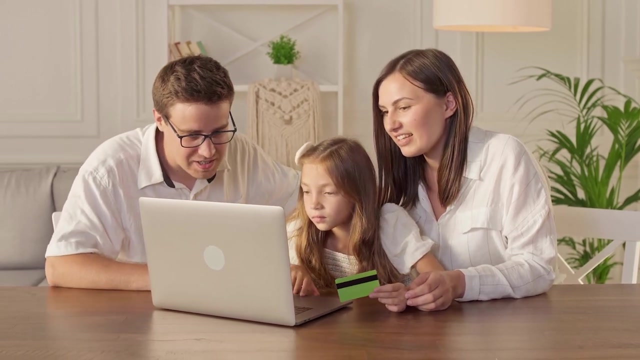 using her debit card and directly access money she already has, which means that her account balance would go from $500 down to $150.. Hmm, that is a lot to think about. Which option would you choose if you were Frankie, And what are some ways that you can use debit and credit cards? 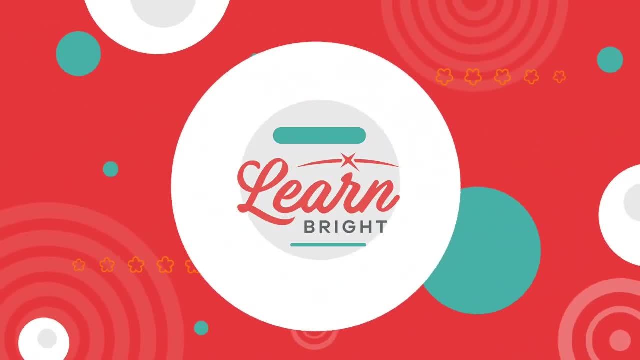 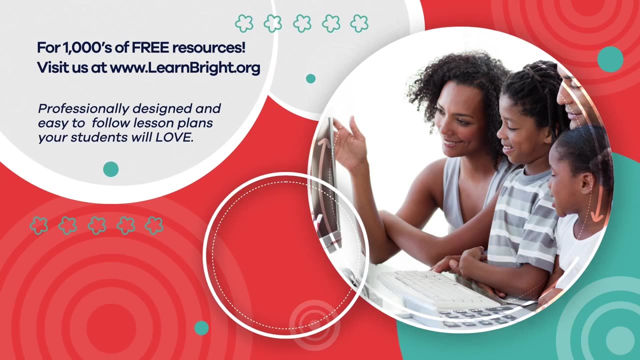 responsibly. Hope you had fun learning with us. Visit us at LearnBrightorg for thousands of free resources and turnkey solutions for teachers and homeschoolers.